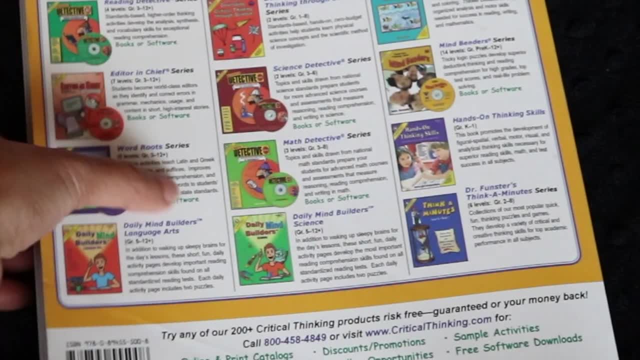 for a long time. I've done similar puzzles to the ones in Mind Benders when I was in Gifted as a Child and I remembered those. So when I saw the book I just knew I had to get it, and fortunately my son enjoys them as well. 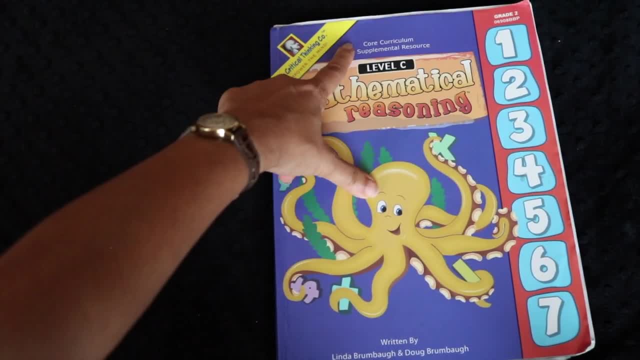 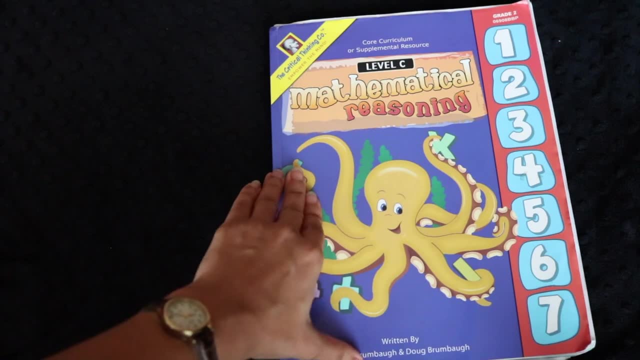 So the Mathematical Reasoning books are labeled as being either core curriculum or a supplemental resource. I believe that they're much more effective as a supplemental resource precisely because they don't have very much spiraling or review or just kind of rote repetition. 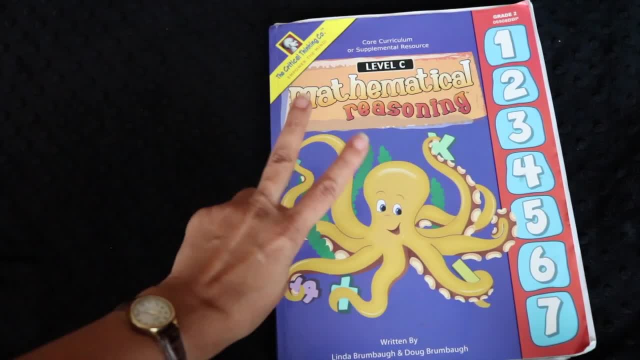 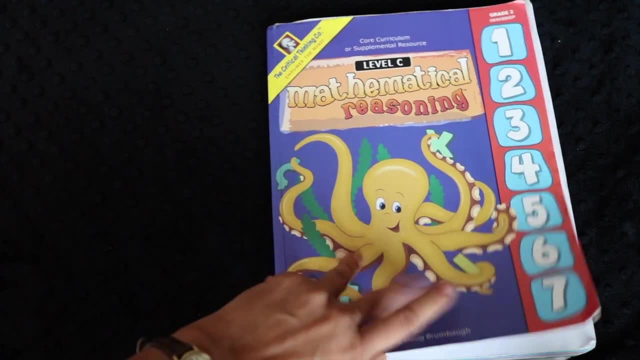 We combine Mathematical Reasoning with Singapore math. Those are our two primary sources for math education in our house. I do throw in the Math UC DVD every now and then because I got it as a sale one day, but we don't do the workbook for that because we find it incredibly boring. 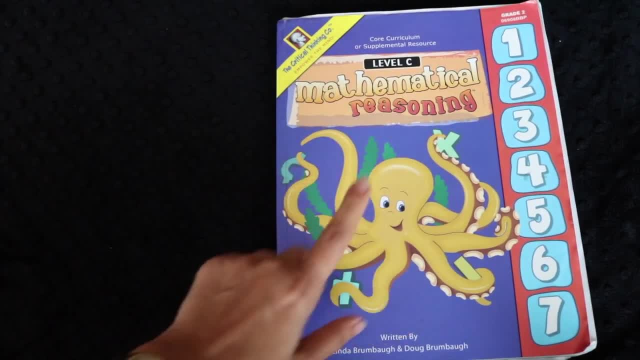 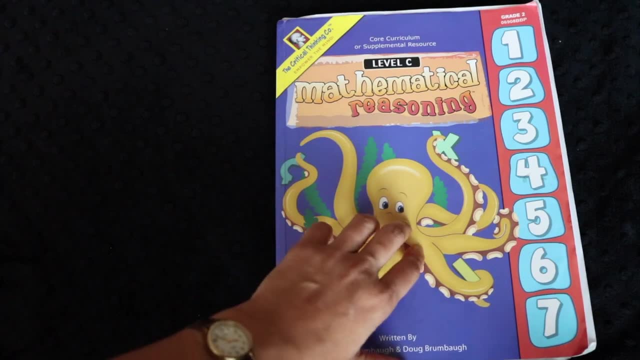 Next year I might incorporate Beast Academy as well, but right now this is really good for us and I think I will continue having Mathematical Reasoning as a supplement for next year as well. The book Binding was not that good in this one, because you can see it's just glued on. 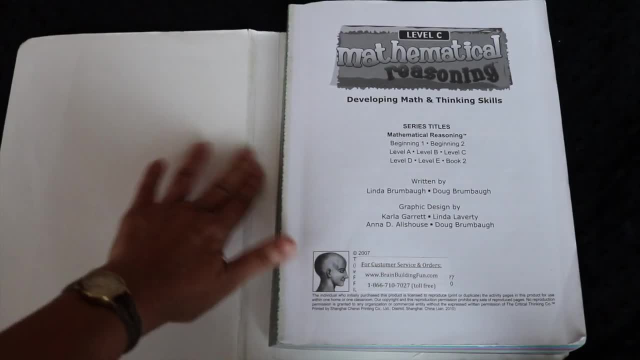 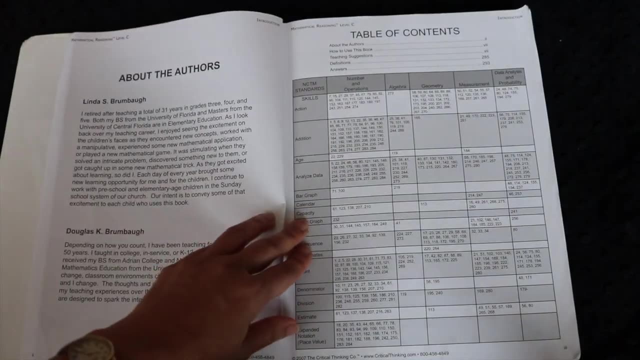 but the pages are staying together really well with the glue but for some reason this binding separated from the cardboard. I think I can just glue that back on, but just so you're aware that does happen. So the book begins with this table of contents and I'll just zoom in to show you that it. 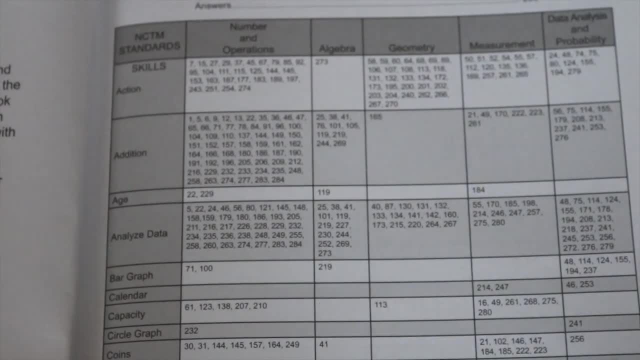 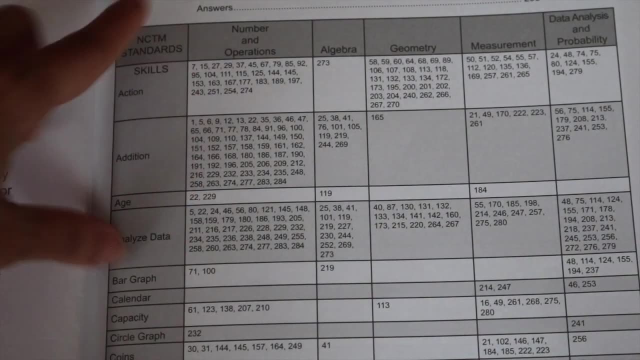 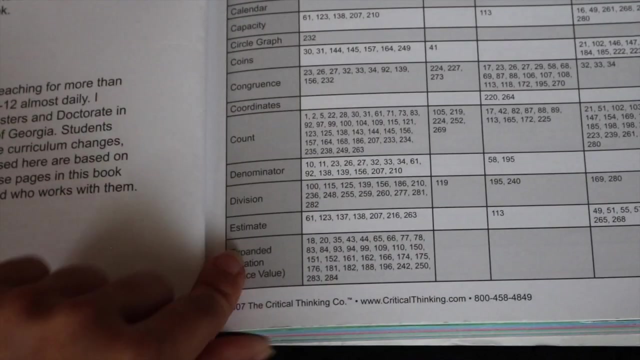 is actually a really useful table of contents if you intend on using this book as a supplement and not marching straight through, because it talks to you about what standards are on this side, in alphabetical order. So it has everything from action to capacity, circle graphs, coins and all the way down to things like expanded notation, and there's quite 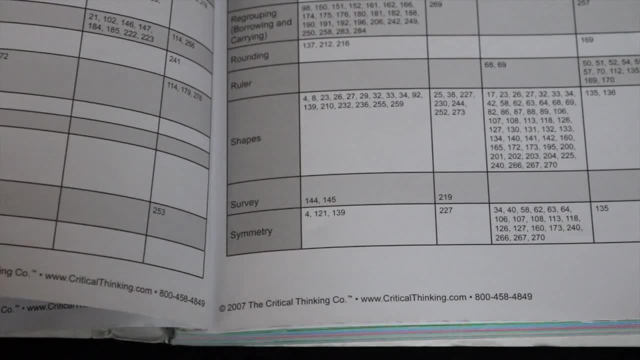 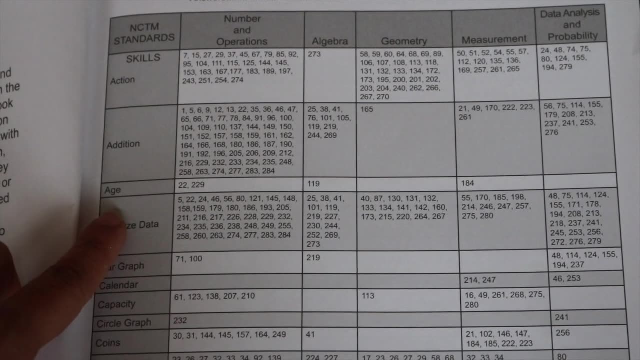 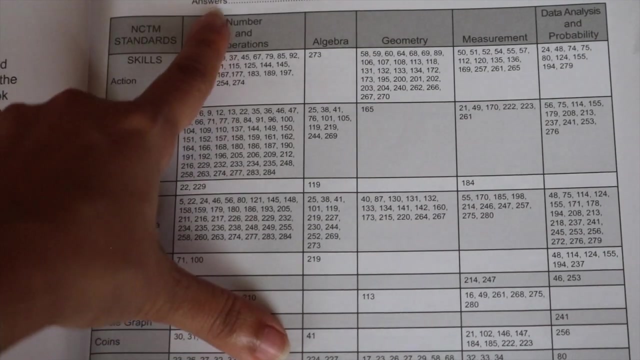 a few pages of contents here and it tells you exactly what pages each of these things are on. And not only does it break it down into different standards- so for example, addition, it'll break it down into different activities for that standard. So addition here is practiced. 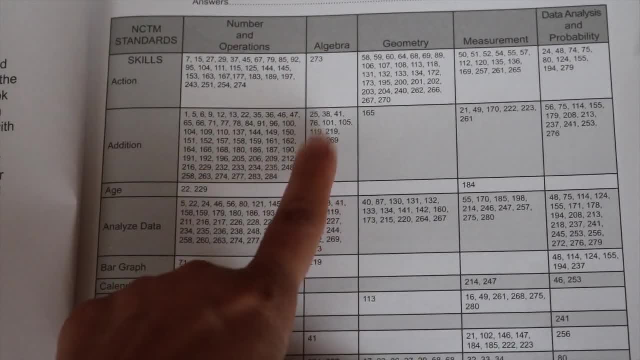 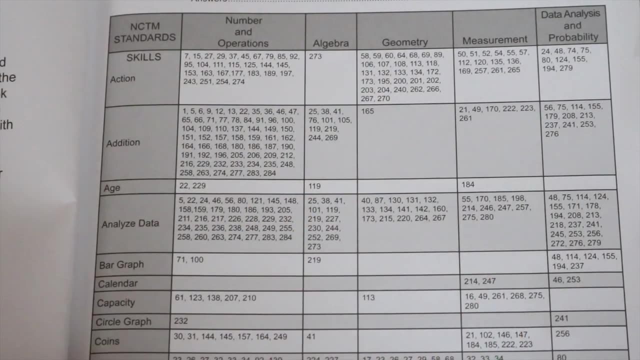 with numbers and operations on all of these pages in an algebraic way, on these pages, in a geometrical way here, Incorporating measurement here, data analysis and probability here. So if you wanted to talk about coins again, here you have just numbers and operations with coins, but then 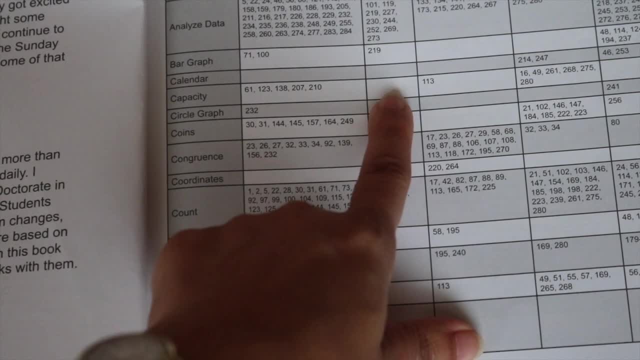 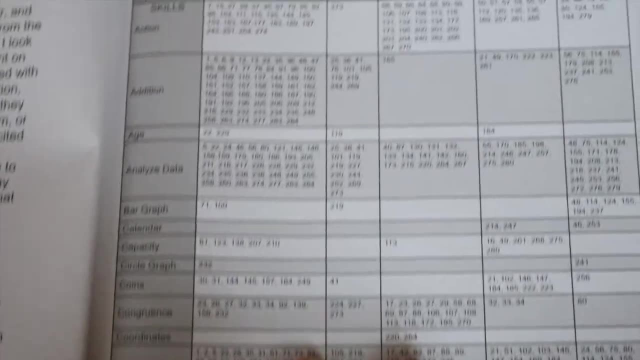 here you have algebra with coins and then so on and so forth. Here you have measurement with coins, and so they do, I think, estimation and stuff like that there, And it's a nice way of breaking down exactly what each page is If you're interested in truly customizing. 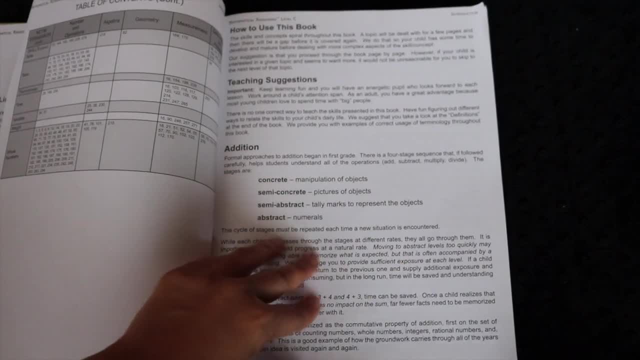 when you do what page, they make it really easy for you. We don't do that, but we do have a lot of different ways to do that. So if you're interested in customizing, when you do what page, they make it really easy for you. We don't do that. 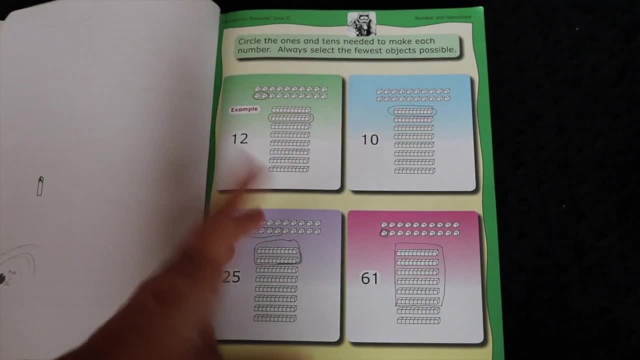 but we do have a lot of different ways to do that. We don't do that, but we do have a lot of different ways to do that. We pretty much sort of marsh through And it's just fun. It starts off pretty simply with numbers and operations, just kind of getting them back. 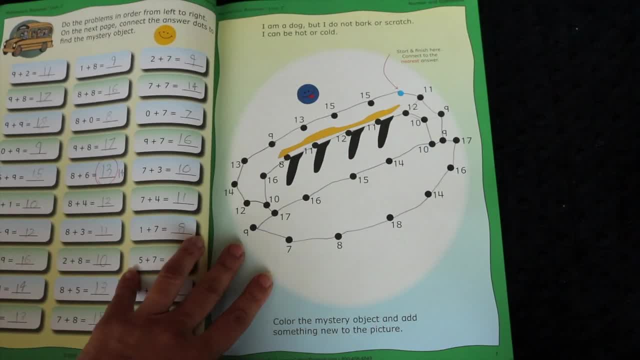 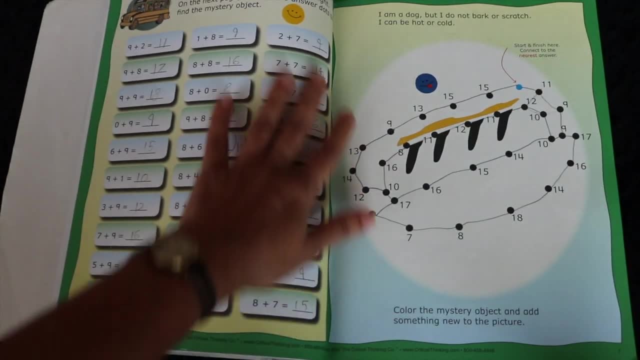 under speed But you'll see each page is quite different. No two pages repeat in this book. This is probably the most commonly repeated activity And it's probably every 20 pages or so, where they'll have one page of numerical operations and then have like a dot to dot. 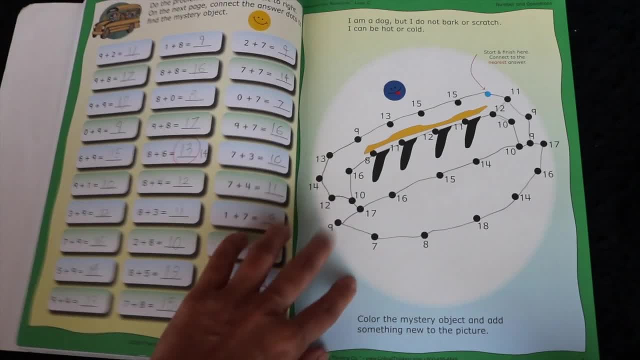 I find this a little bit irritating, And this is the only thing I find irritating about this book, because this dot to dot is so rare. I think that's what they serve you best, because this is a nuts to nuts class. Sometimes, if you coloured with numbers, you'll spend 했. 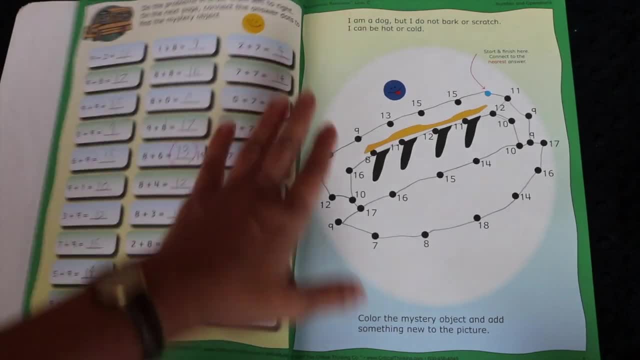 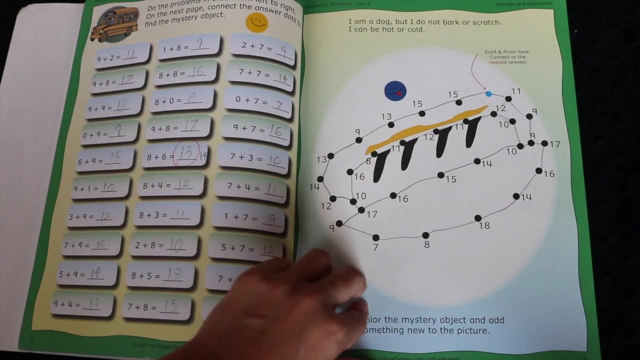 makes it often, sometimes easy for them to fill in the answers. So when we do this, I generally put in a piece of construction paper here, just so he's not tempted to follow along and fill in the answers, and it works out pretty well. 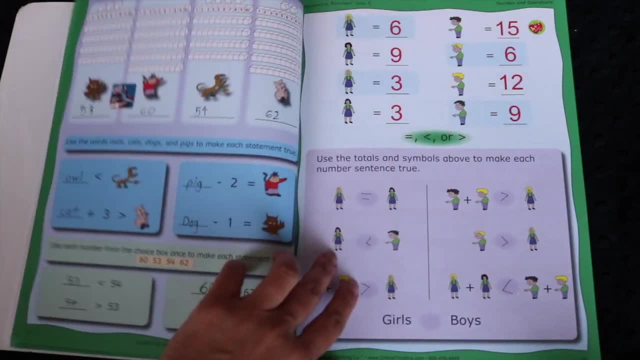 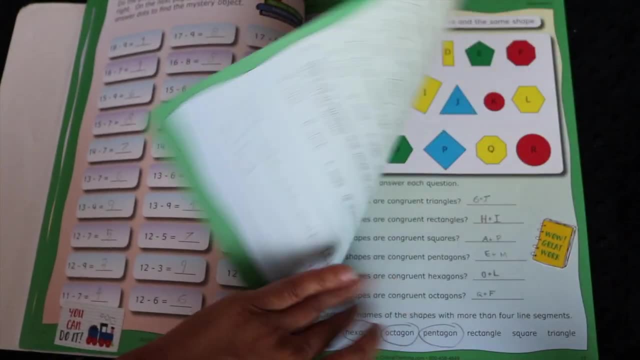 As you can see, it does things for equal signs. I like how colorful the book is, but the pages are not glossy, so they're really easy to write on with pencil, which is nice, And it just keeps marching on straight through. 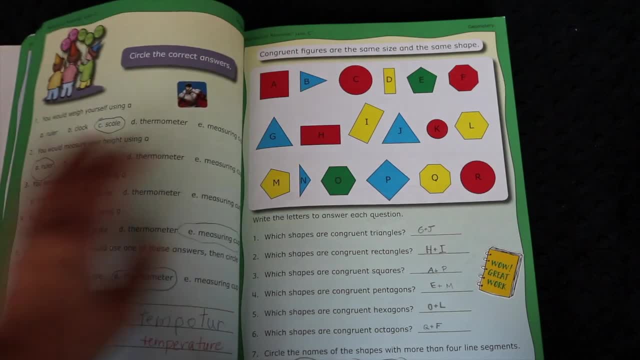 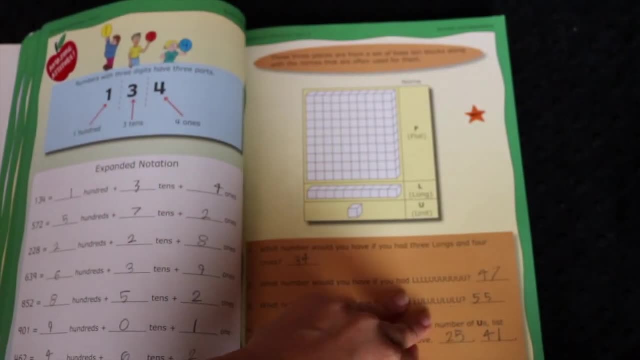 So here you'll see, at the top of the page it rotates and tells you exactly what the page is addressing. So here it says geometry, and on this page it says numbers and operations. Here's another numbers and operations page. Here's an algebraic page. 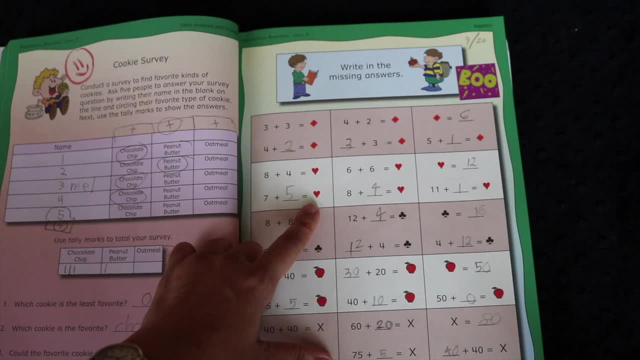 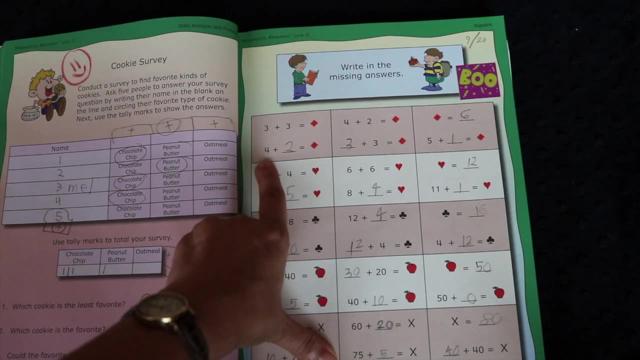 These types of pages I find really enlightening for a child and really good practice for algebra to come, because it's teaching them the concept in a very simple way that you can have a symbol stand in the place of a number, which is fundamentally what algebra is about. 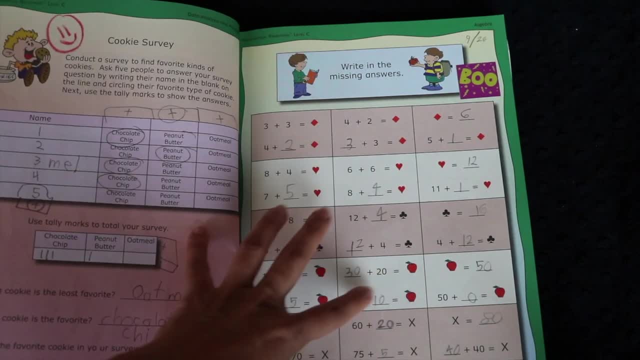 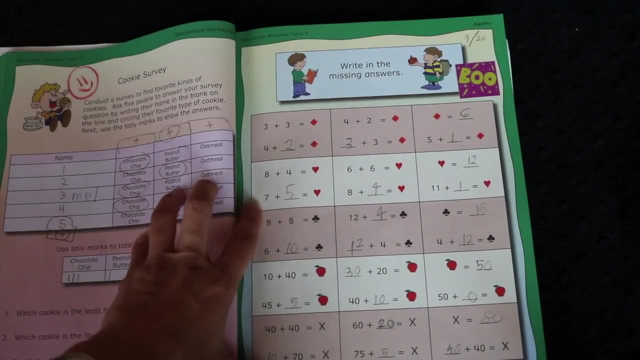 I had friends who started doing algebra in eighth grade and could not grasp that concept that x could equal a number. And here they're teaching you it very simply by saying that here you're gonna have 12 equal a heart. See, you can have eight plus four equals a heart. 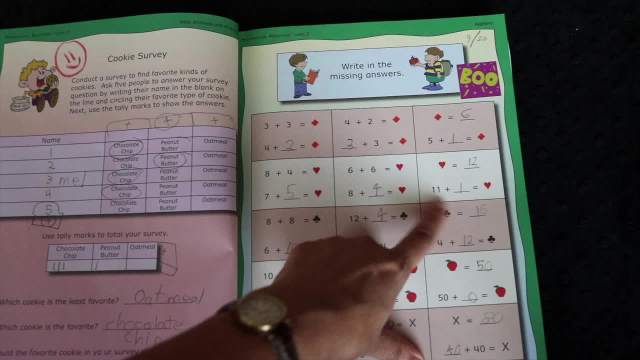 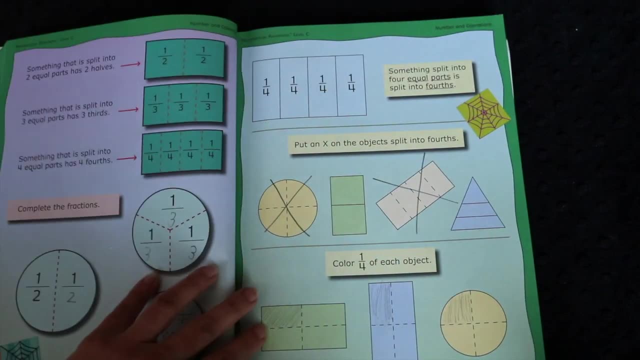 or you can have seven plus five equals a heart, And then later, if you have 11 plus blank equals a heart. what will it be? What does the heart equal? It's teaching them algebra without teaching them algebra, if that makes sense. 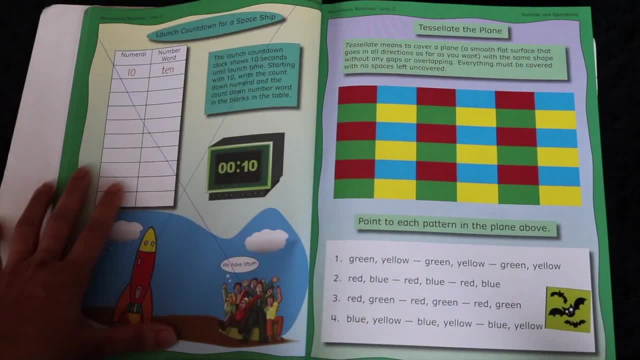 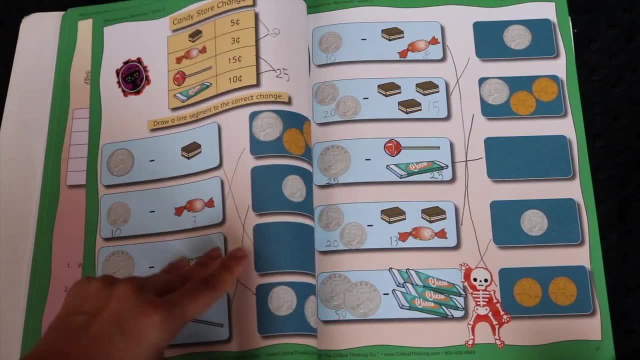 It introduces fractions in a really graphic way- Pages that I don't think we should do or that I think that are a waste of our time. I just cross out and he just moves on. I like how they have activities like this that introduce concepts like tessellation. 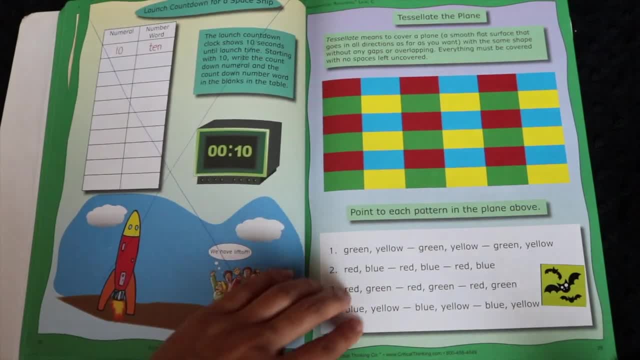 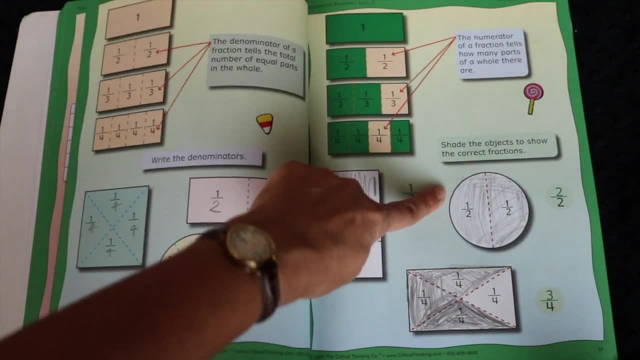 and actually have an activity as well. So here you had to find the patterns in the tessellate. There's other ones where you have to put your finger down on a page and you do a probability exercise with that, So really fun. 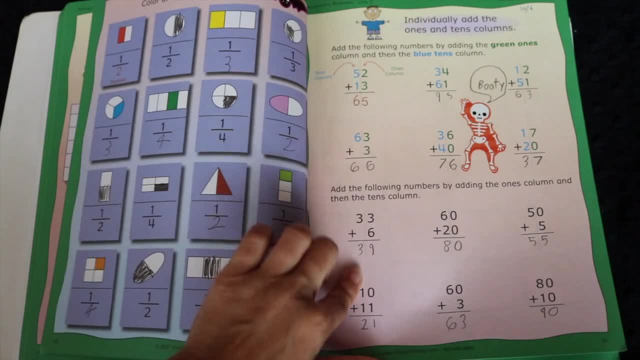 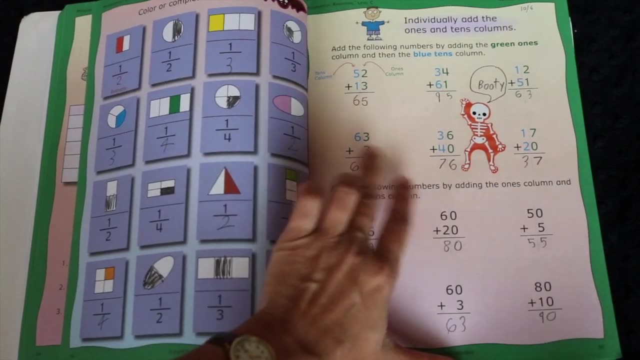 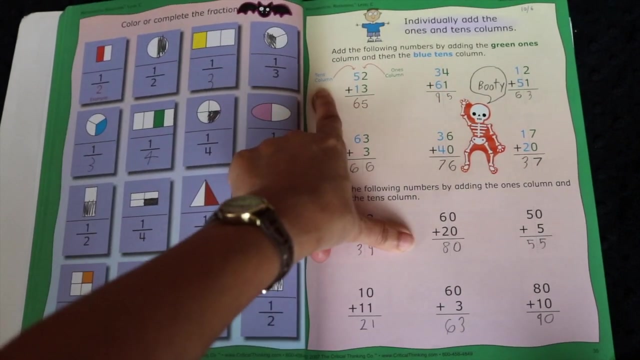 I like how it teaches them addition in a very simplistic way, And it shows you one's column, ten's column, and keeps them in different colors. So there's many different ways of approaching a learner in this book. Not only do they talk to you in actual words, 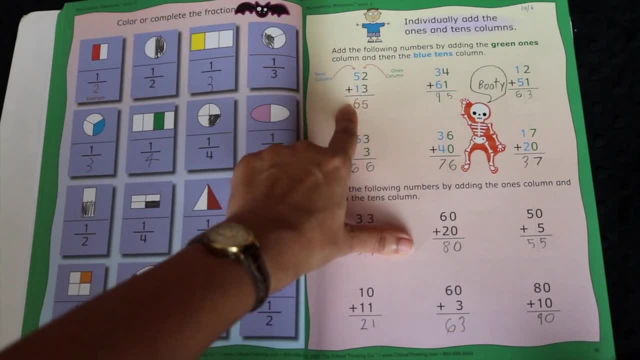 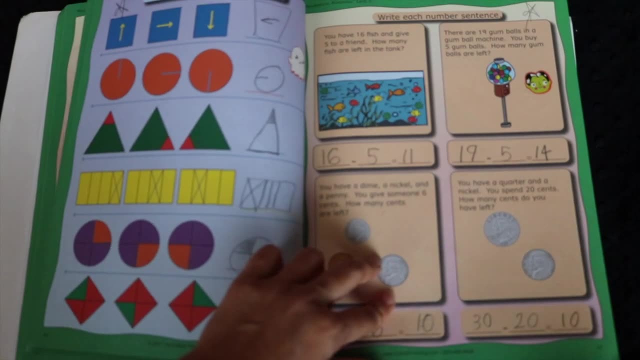 for those that like clear labeling, they also talk to you in colors. for those that are more visual in terms of learning. They incorporate fun activities in the midst of less fun activities. When they show coins, they show you the actual picture of a coin. 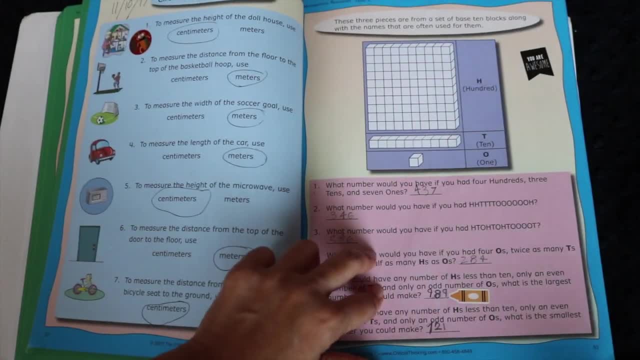 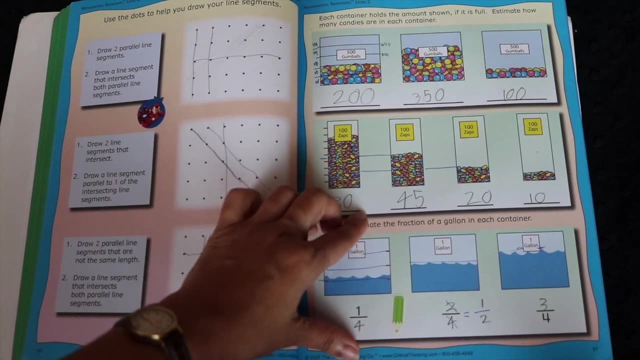 which is another feature that I appreciate. And it goes on and I'll just flip through for you just to show you some of the pages. The estimation pages are very valuable. My son has difficulty with estimation sometimes because a lot of times when they'll see it, 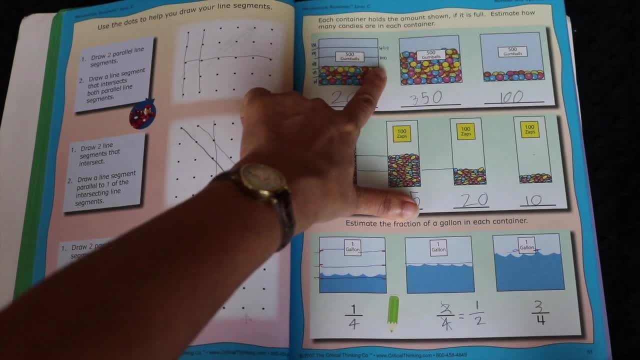 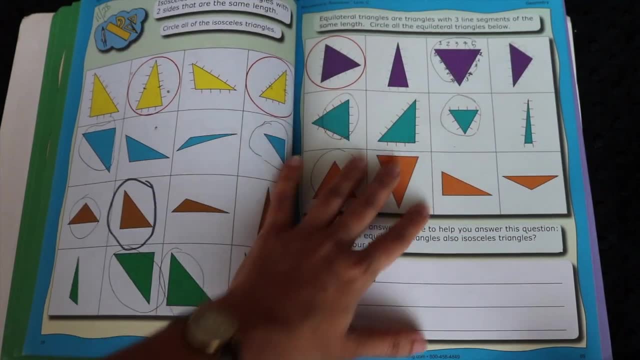 it's actually very precise Here, you'll notice they only provide the lines in one of them and then the lines disappear, which makes it a much more realistic estimation activity. They have a lot of geometry in here as well. Very simple concepts introduced in, I think. 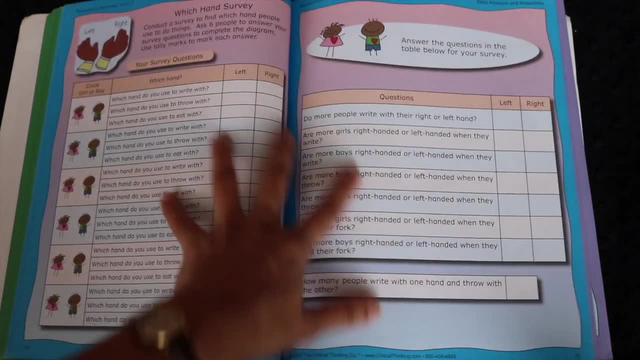 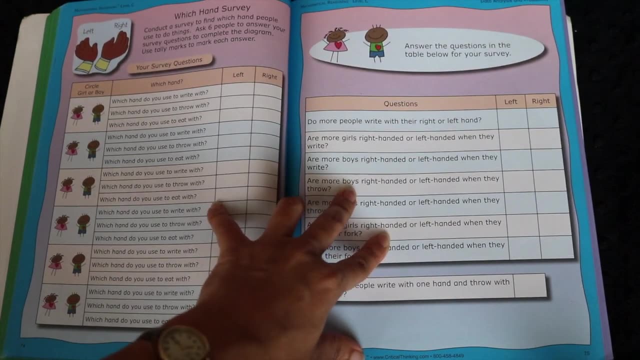 exactly an appropriate fashion for this age group. There's surveys in this book as well, and we generally save the surveys for when we do school in a coffee shop or when we're going to the park And if I happen to have this book in the car with us. 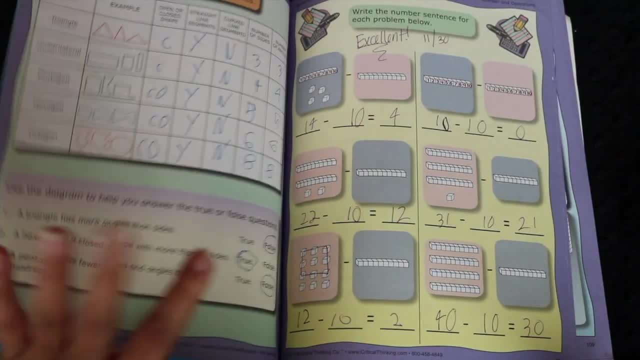 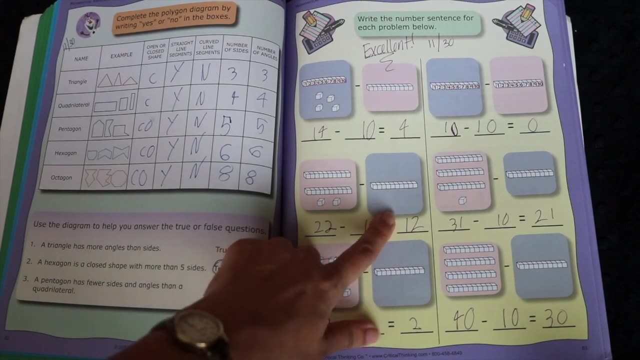 then we'll take it out and he'll run around and interact with people and survey them, which is really fun, And we just go through. It'll incorporate little blocks and cubes. So if you are doing this in conjunction with MathUC or a curriculum that incorporates 10 blocks, 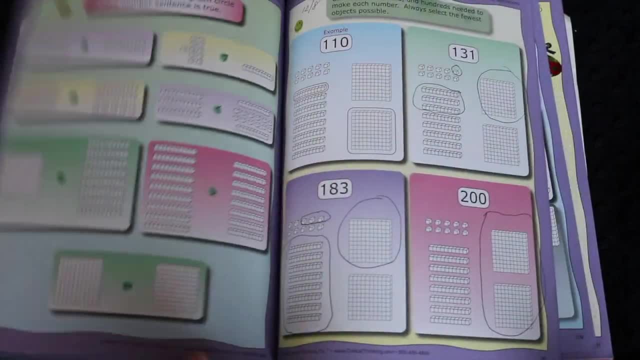 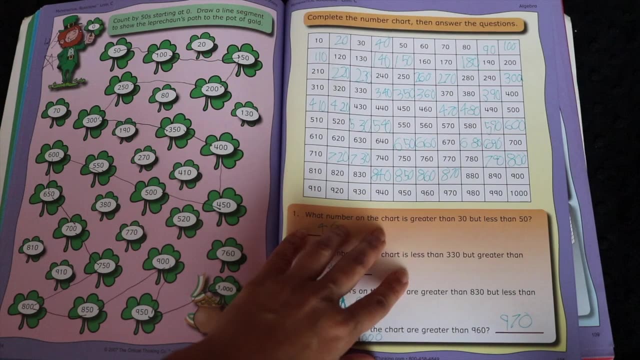 this will be a good supplement to that as well, because they'll be familiar with that idea. as you can see here, for MathUC folks It's very similar. They do a lot of work with number charts as well, just to teach them. 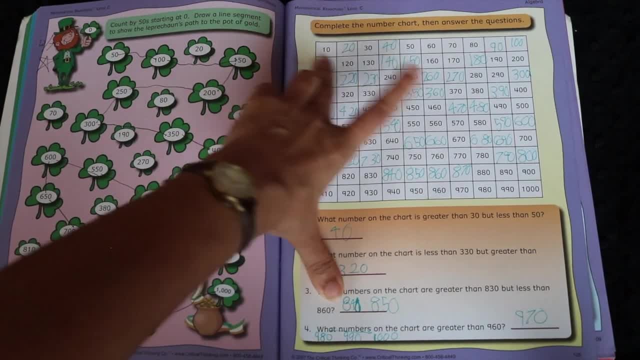 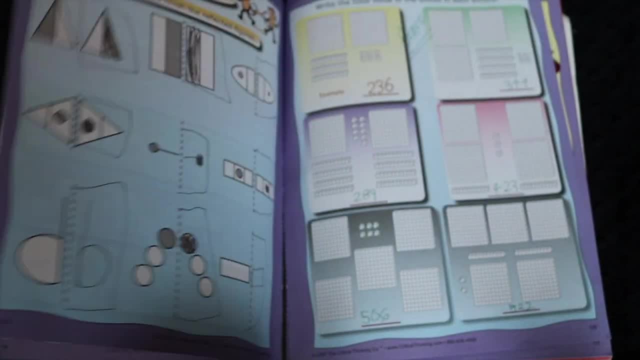 If you'll notice, here it's not a hundreds chart, It's a 10 to 1000s chart, So it teaches them relationships of numbers that you might not often see in a second grade curriculum. They deal with issues of symmetry and reflections. 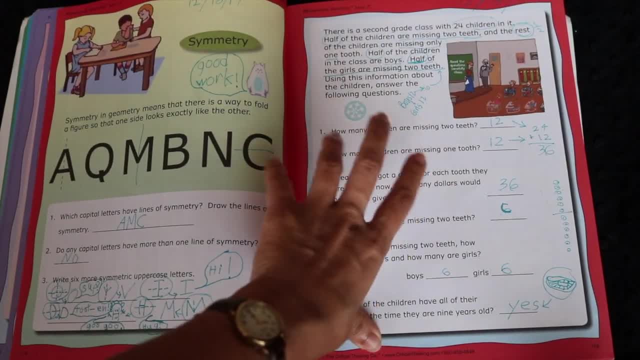 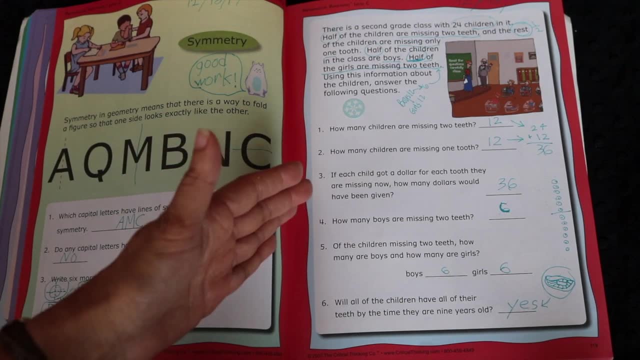 This was a particularly challenging page that we recently did And it's a word problem but based on what they say here, you have to figure out the answers And it's a little bit tricky. We definitely talked this one through, but it was fun. 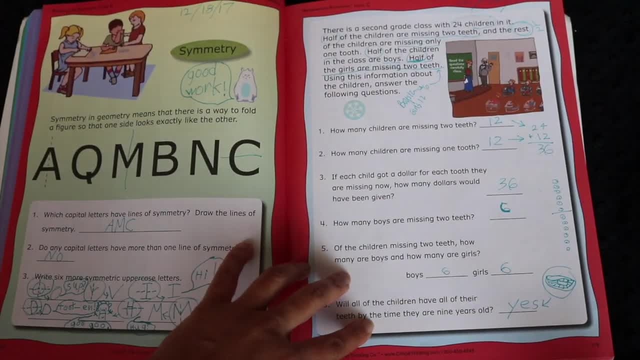 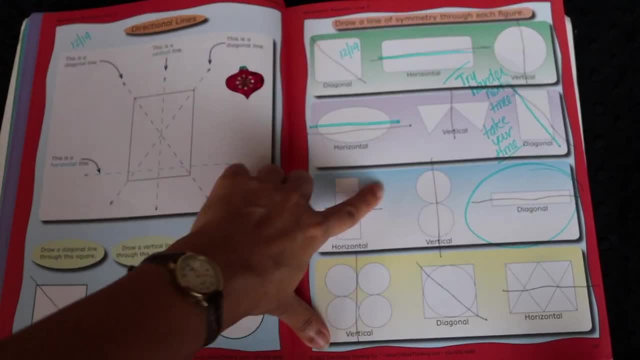 And we had the opportunity to talk about how we would work through a more complicated word problem. I like that the book does not dumb it down, Although they will repeat things many times. you will find a variety of activities and it's a really good way of pinpointing. 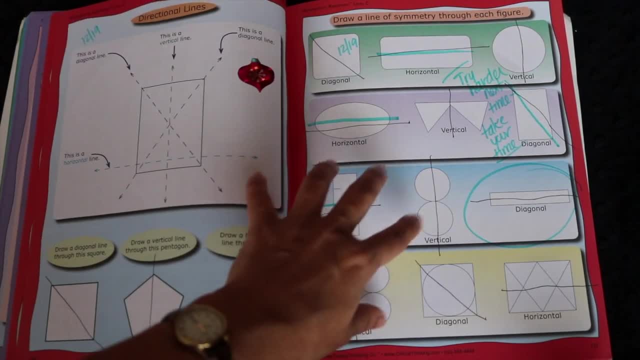 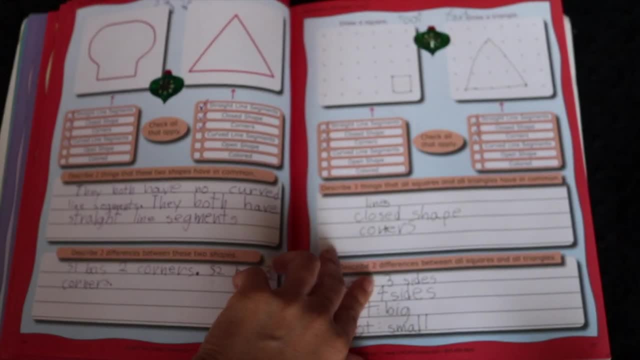 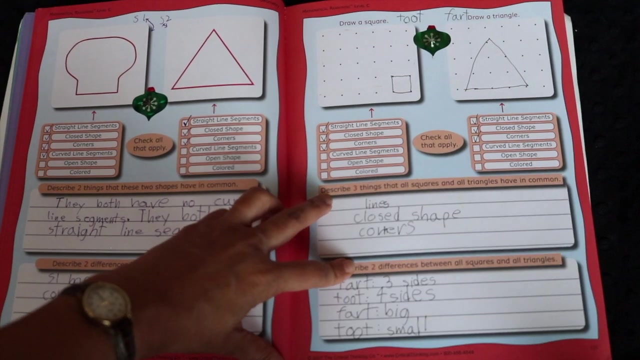 mathematical concepts that your kids might not be so comfortable with, that you took for granted, For example, estimation or word problems. Here is geometry again, and they take them through the steps of actual proofs. So when later in high school they take geometry, 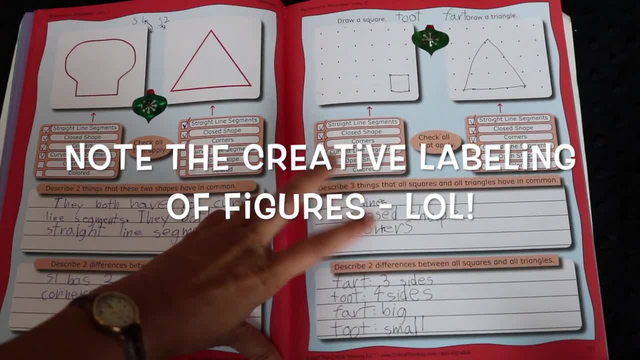 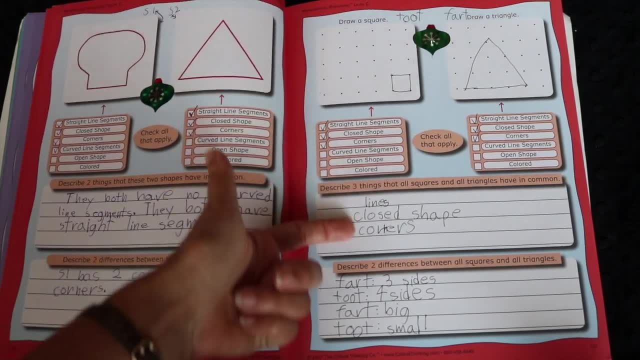 they will have to do proofs by saying, like: why is this thing that you already know to be true? true, Like, what is your logical reasoning? And they do that with them, where they ask them to describe things that are the same between different polygons. 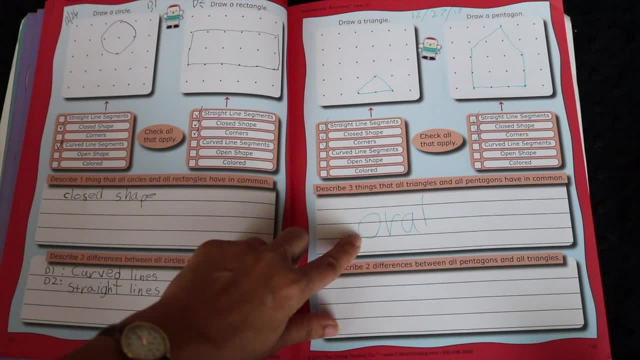 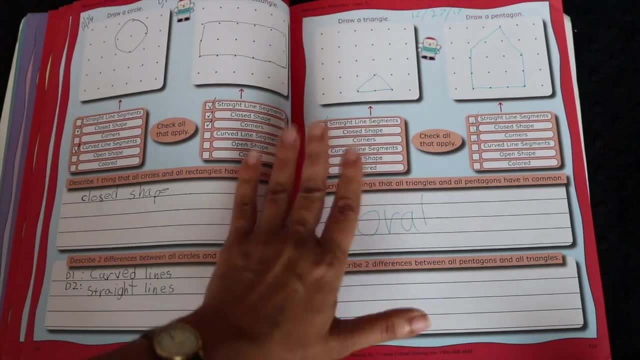 and things that are different, And I think that's a really good exercise. Sometimes, if you'll notice here, it says oral. Sometimes, if my son is feeling like he doesn't want to write all of that down, I simply ask him to explain it to me, and that's perfectly fine. 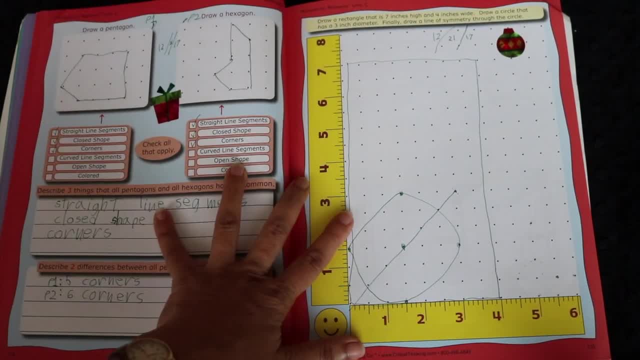 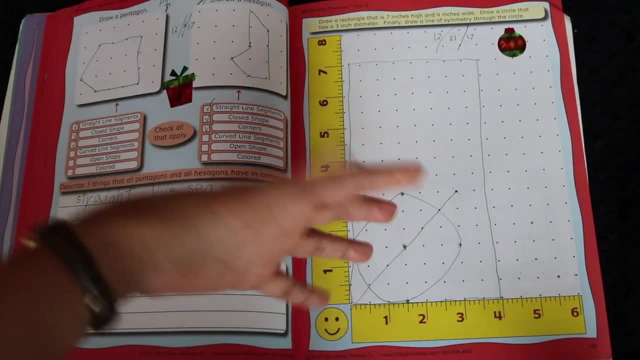 He gets to write the word oral and we move on. That's a really good way of keeping your child's interest and not making them resist you with an activity that you know. really, what are we learning here? I want him to be able to do the proof. 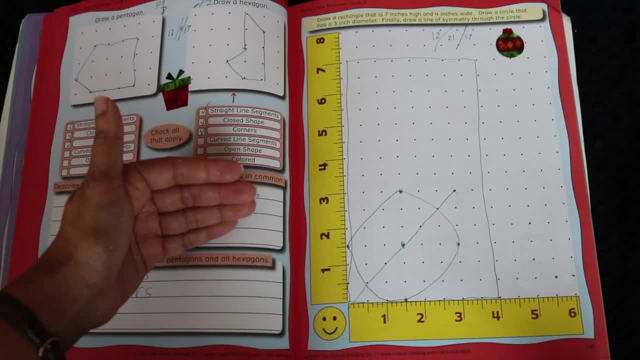 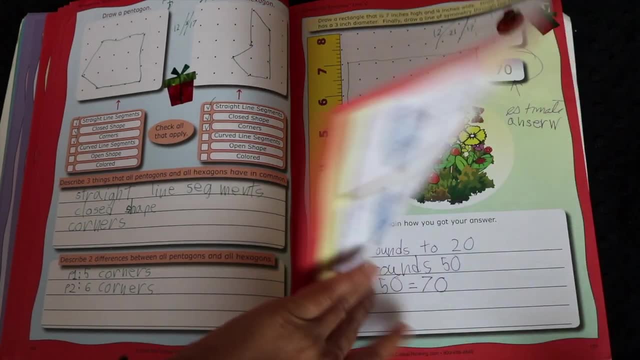 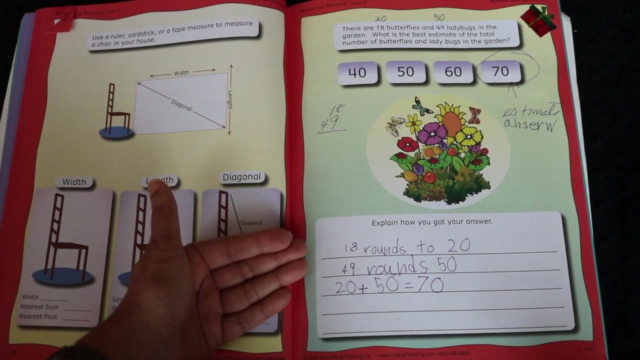 This is not a writing exercise, So if he is feeling like he does not want to write at that time, I'm going to let that slide. That's a good tip for all of you who have children, perhaps, who want to move through things and don't feel like doing one particular aspect of an activity. 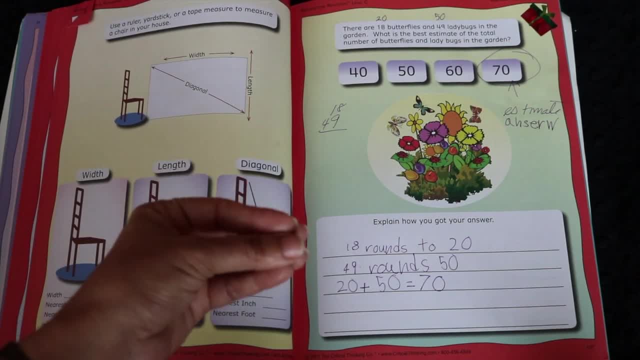 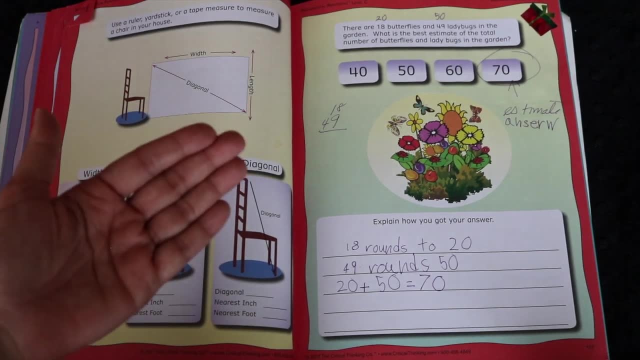 Ask yourself whether that's actually the point of the activity. Is that what you want your child to learn from that activity, If it's not? try to accommodate them? It truly doesn't cost you anything and it probably brings you closer and it shows them that you are listening to them. 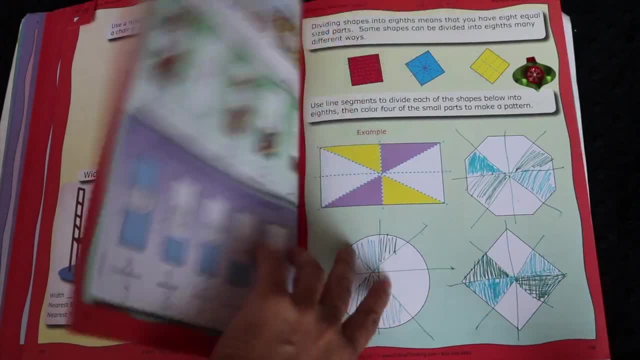 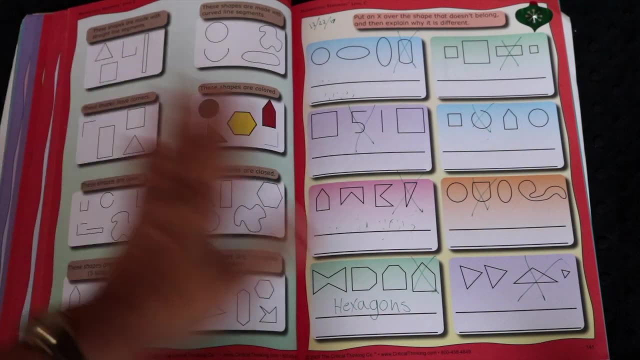 Anyway. so here's a good estimation activity And you know some of the pages take much longer than others, which is another thing that makes it a good book to use as a supplement, because if you just want to do a quick activity, 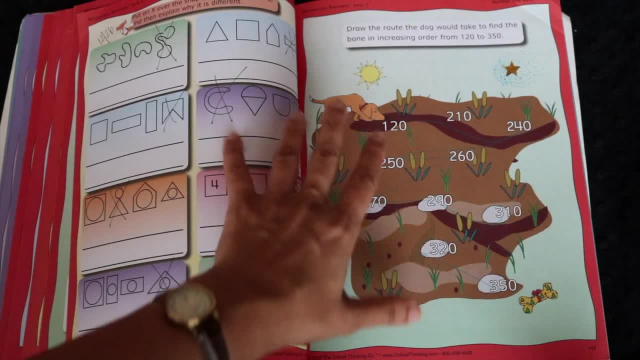 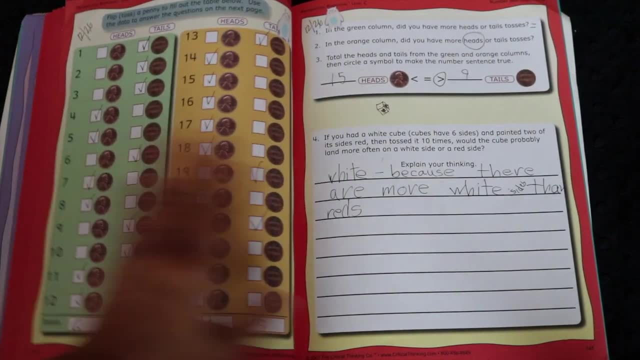 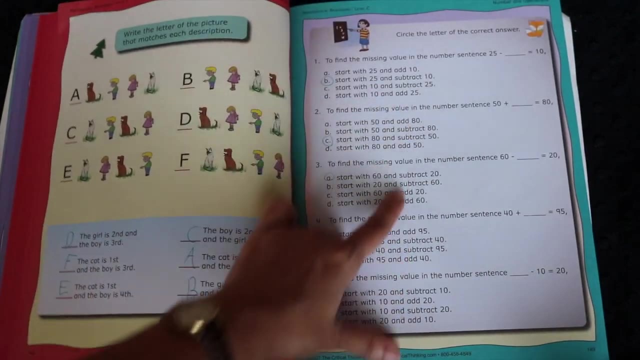 you can definitely skip ahead a little bit or skip around and find something that's only going to take a few minutes. For example, this activity took about one or two minutes, whereas something like this again would only take a little while. but something like this takes a little bit longer. 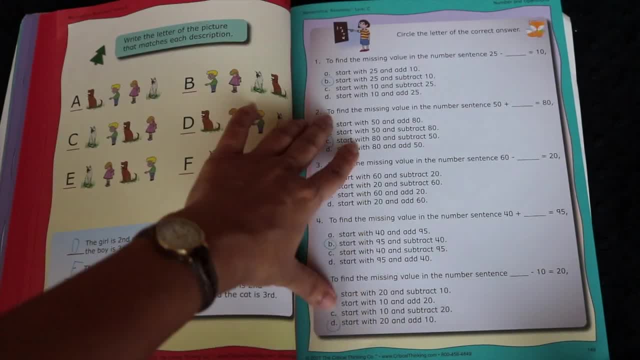 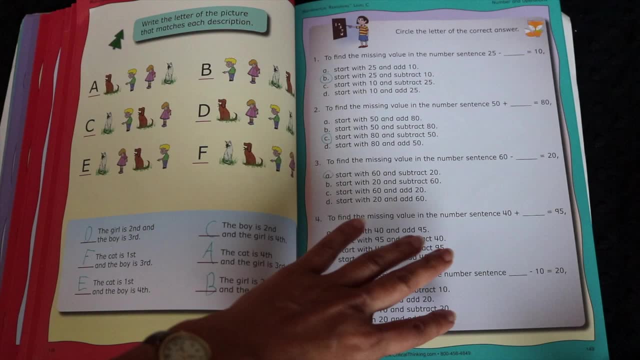 because it involves more thinking. A page like this reveals a lot about how your child is processing math. How are they thinking about what math actually means? What are you doing when you're doing a math problem? I really like this book. I cannot recommend it highly enough. 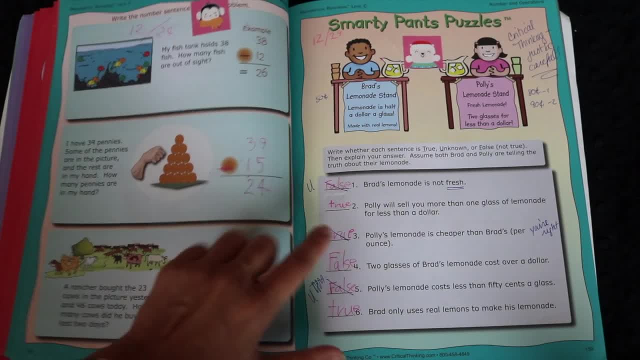 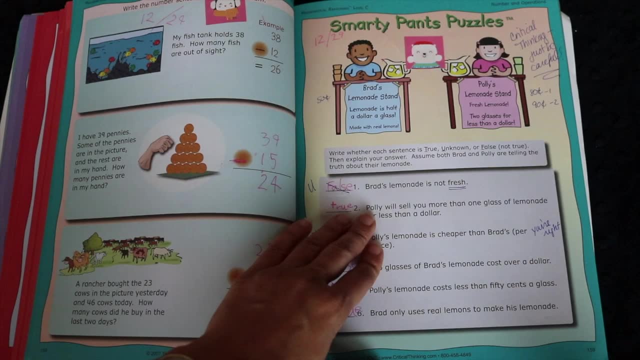 This picture was really, really challenging for him. So we had to talk about how there are things that will be unknown. That concept of being unknown was something he had not worked with before. That things might be true, false, or you might have no way of knowing. 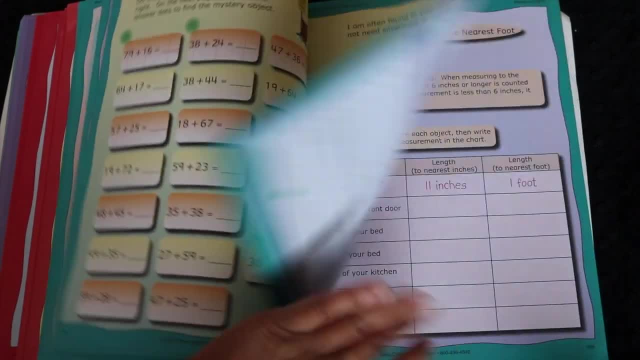 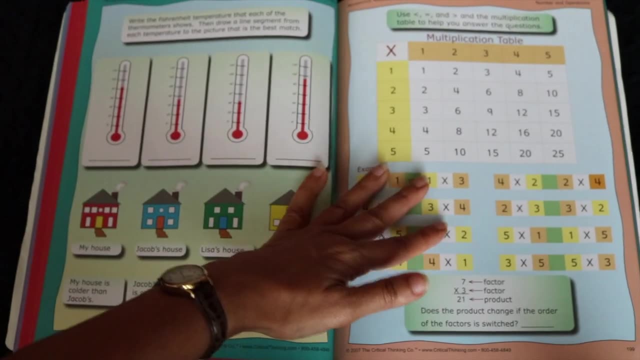 These are the types of things that I found that this book provided, that we really haven't seen in other books. For the most part, I find most of the activities in this book really, really worthwhile. You'll see here around three-fourths of the way through the book. 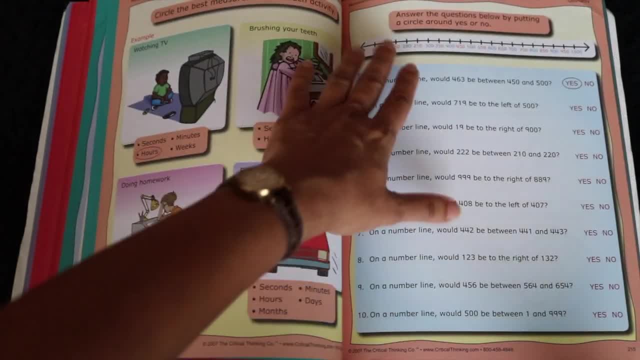 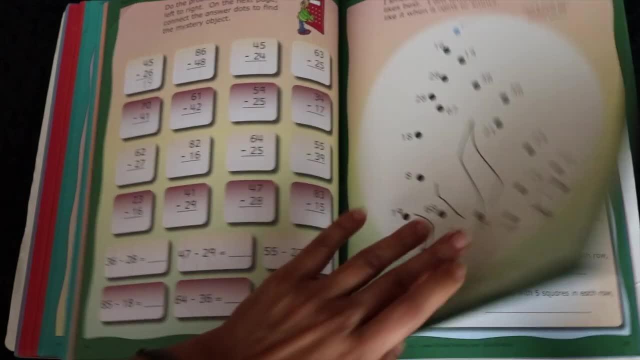 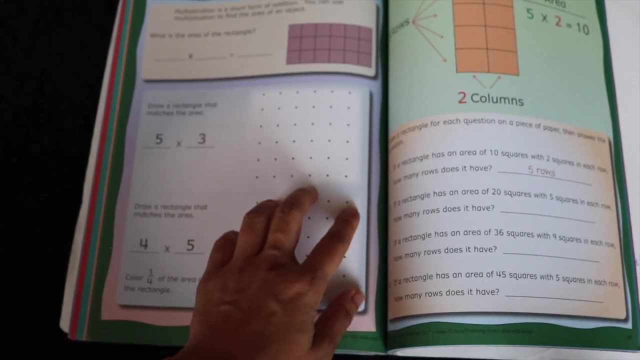 it starts to get into multiplication and multiplication tables. I like that they work with bigger numbers so that we're not always working in the hundreds. They do do time activities scattered throughout, but not too much. I like here that they relate multiplication to what it actually is. 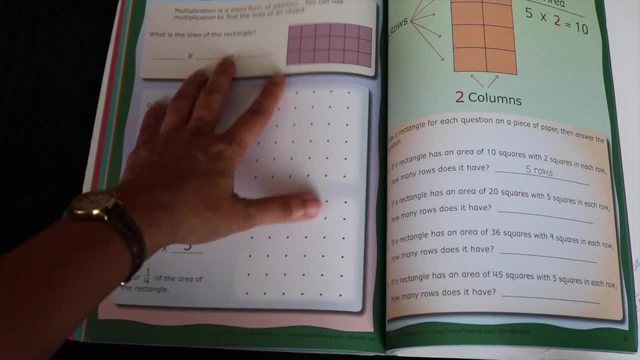 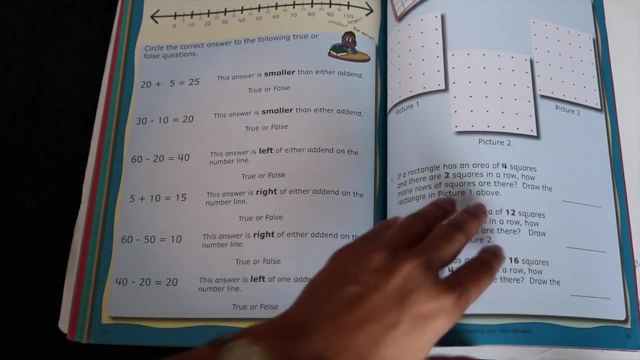 So it'll show you like, draw a rectangle that matches the area It's already teaching your child. that area is related to a multiplication problem, so that this concept doesn't come up later in a completely unrelated way. I really can't say enough good things about this book. 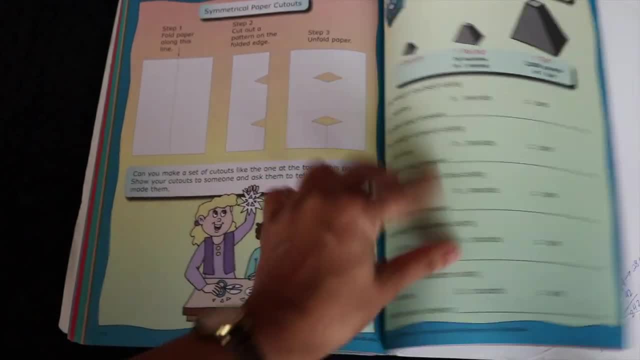 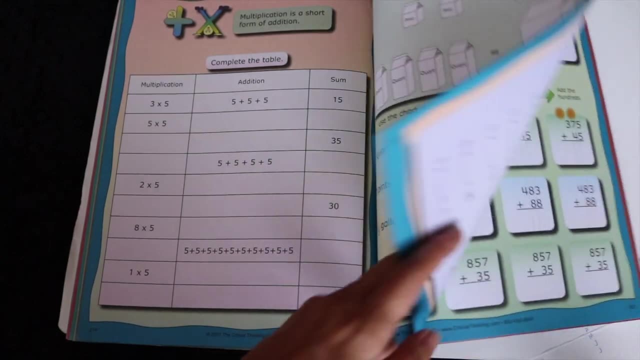 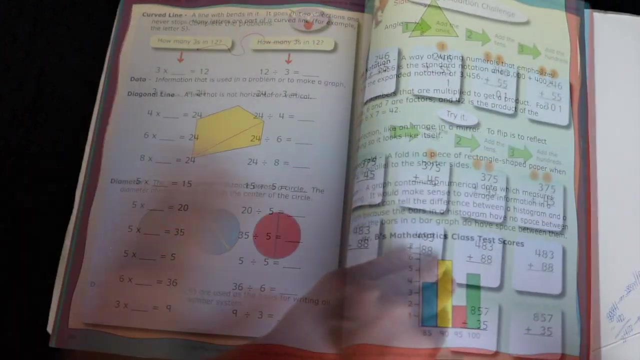 Here it has interactive things. So we're making snowflakes here and it'll teach you about symmetrical shapes and what's actually happening there. So there are interactive activities, there's measurement there, and it goes on throughout. Here it has some three-digit addition and at the very end of the book 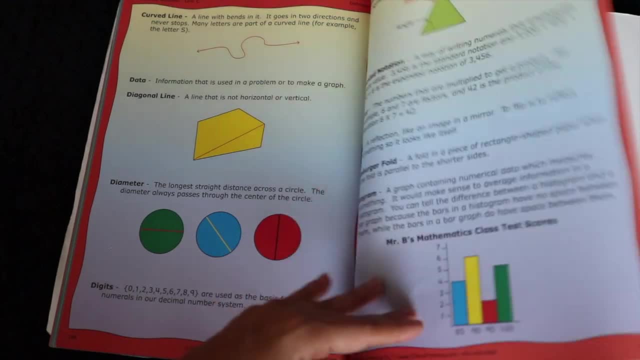 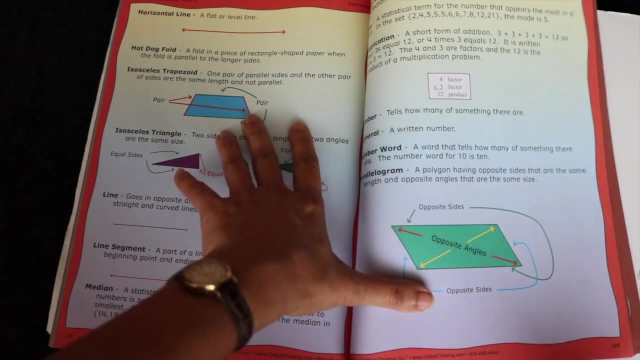 it has a glossary, So if you want to show pictures of what a diagonal line is, what diameter is, what digits are versus numerals, isosceles triangles versus an isosceles trapezoid- I was actually going to. 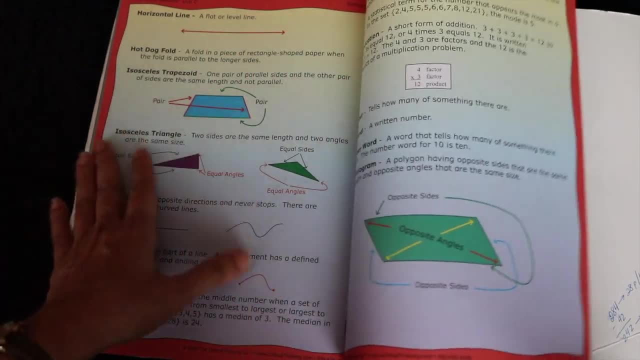 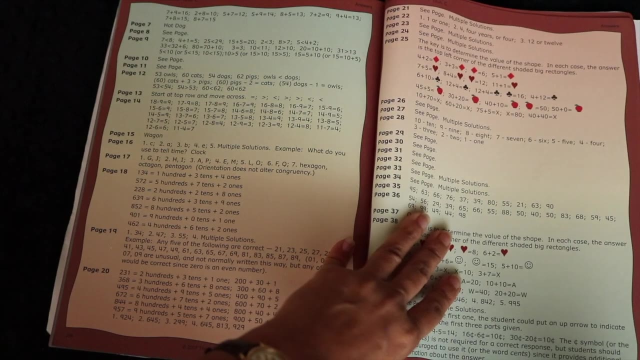 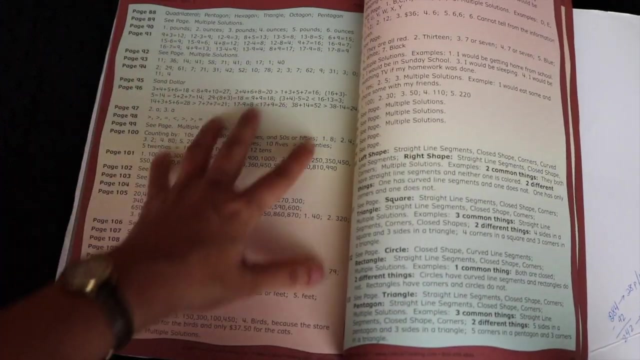 take these pages out for the glossary and keep them in his binder for next year so that he always has something to refer to. At the very back of the book you also have an answer key. So if grading or having multiple children and just not enough time to do all this, 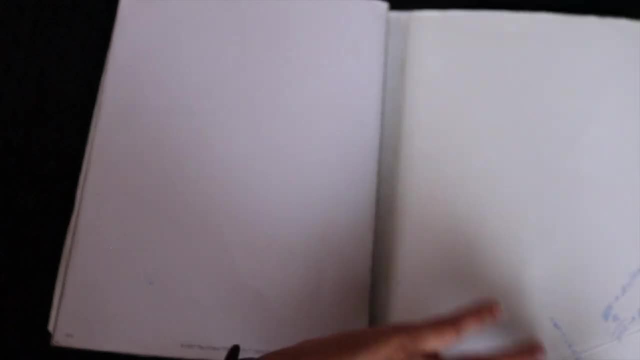 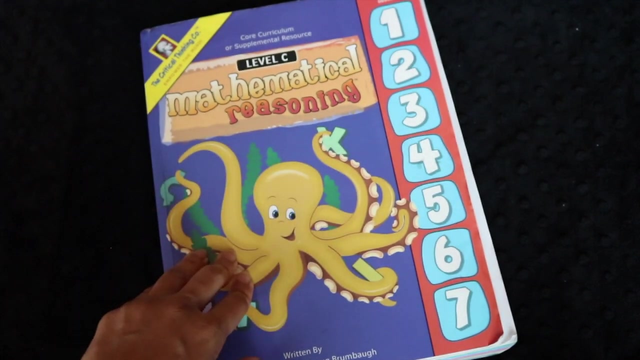 is an issue for you. you do have an answer key in the back, which is something my son has yet to discover, so I don't worry about it at all. I love this book. I cannot recommend it highly enough. If you're looking for a good supplement to round out, I would recommend this book. 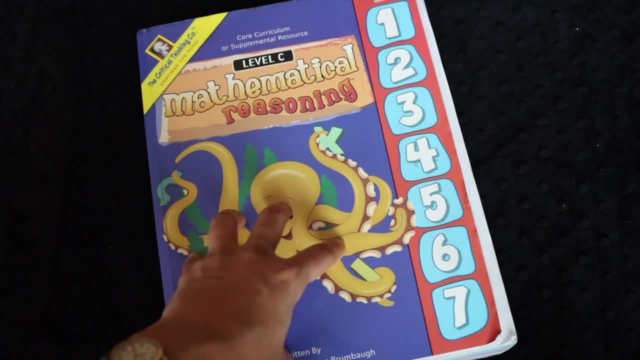 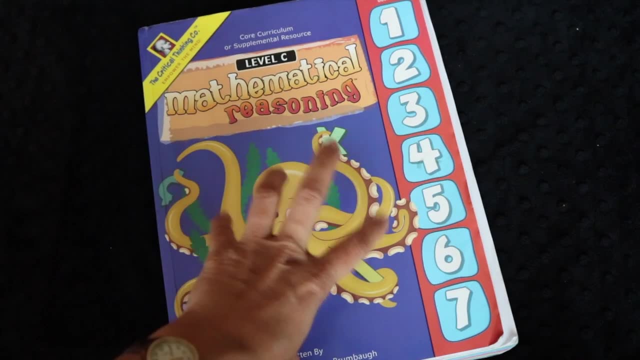 It's a great book. It's a great book. If you want to round out your child's arithmetic education, this is a really good option. It really incorporates a lot of algebra and geometry and money skills into your child's learning. So this is a really really good book and worth the money in my opinion.